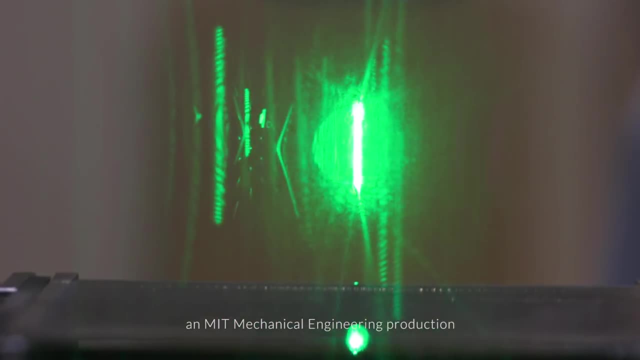 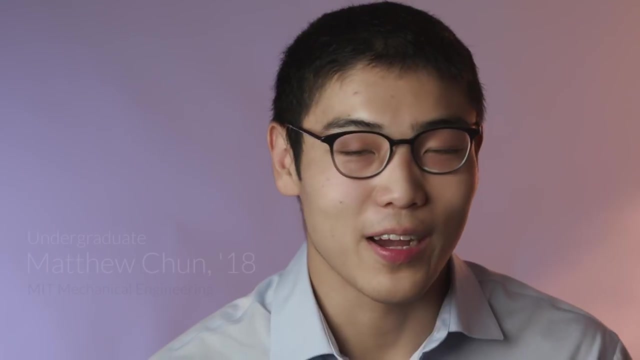 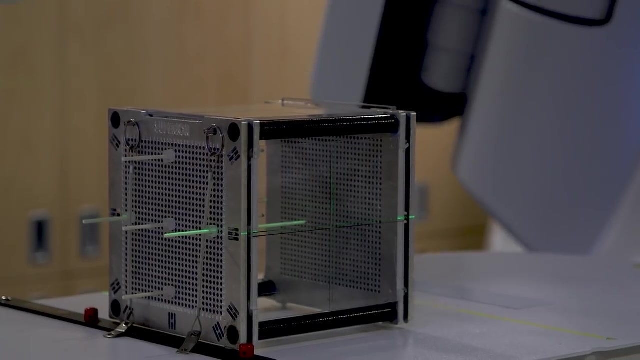 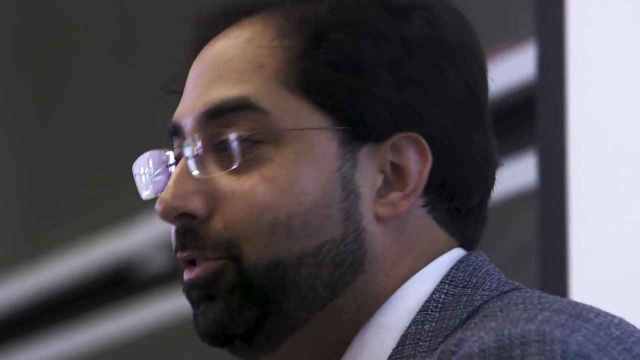 Medical devices are something everybody's going to need and want to have. better Growing up and seeing my grandparents get older and sick, I really wanted to find ways that I could help improve their lives and make them healthier. This course focuses on preparing students for the biggest industry in the United States. Healthcare provides incredibly complicated challenges. 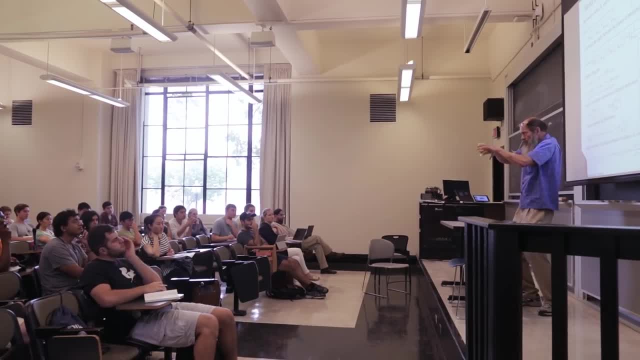 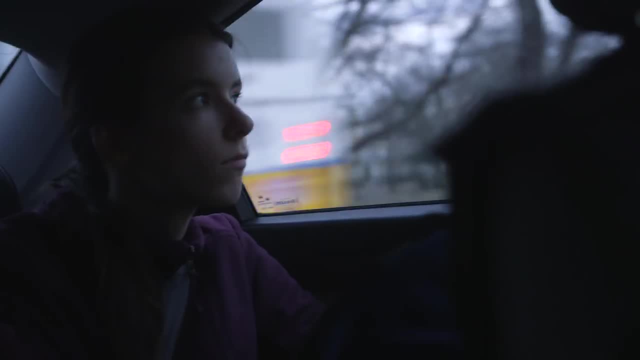 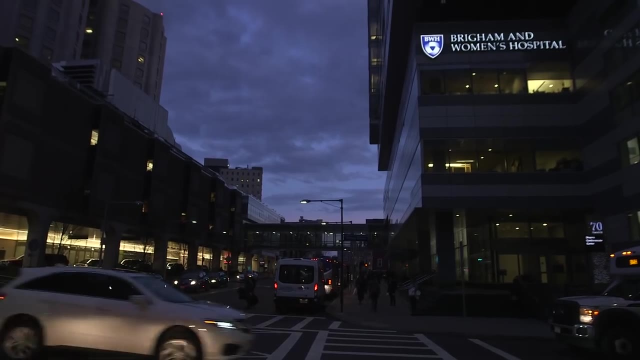 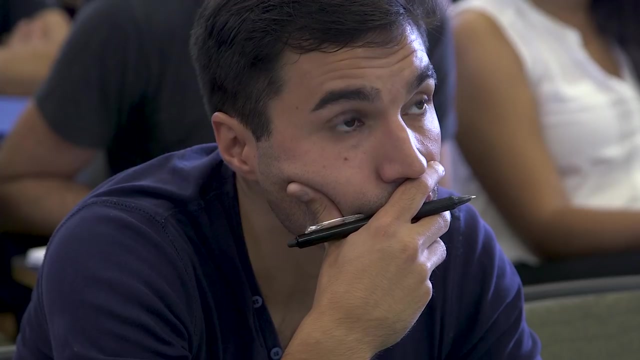 And we teach them how to design a medical device so it's better, cheaper, doesn't hurt so much. I think what makes this class really stand out is its bridging together of clinical practice and engineering principle. We invite a dozen or so clinicians to come in at the beginning of the class and describe. 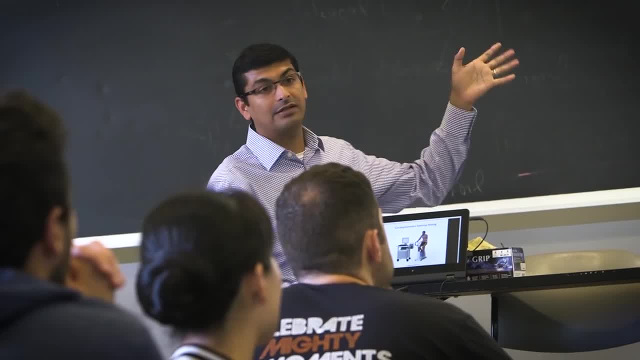 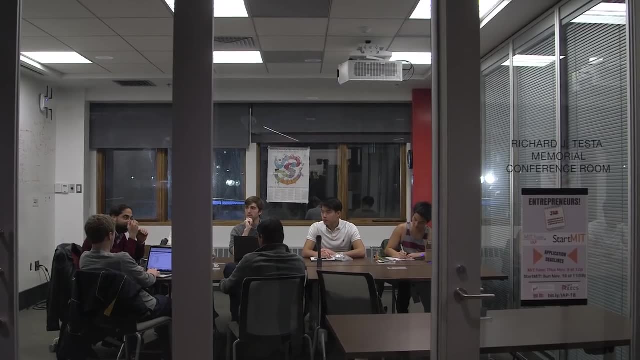 I need a new type of splint, Or I need to create a new thingy for treating this? We are very used to using medical devices in a clinical environment And we often have ideas on how to optimize or change the way they operate. 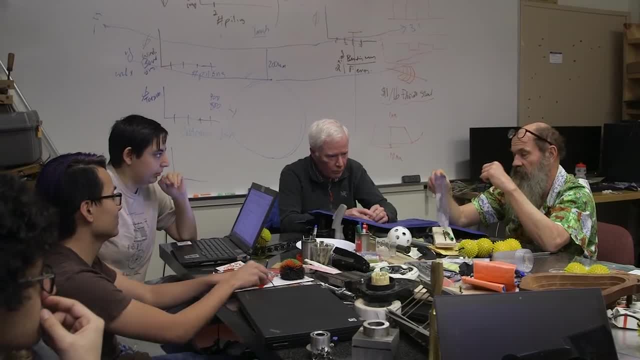 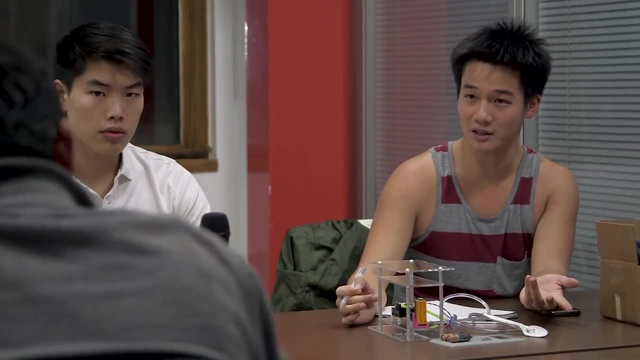 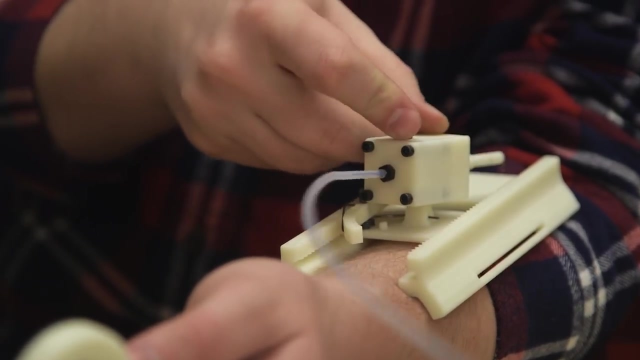 The problem is that we cannot change the filter here. What we want our students in this class to do is not hack and try things at random. We want them to design and experiment thoughtfully. At the end of the 14 weeks, you have to deliver a prototype. 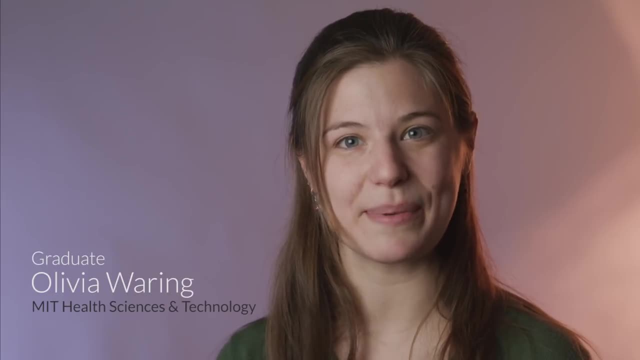 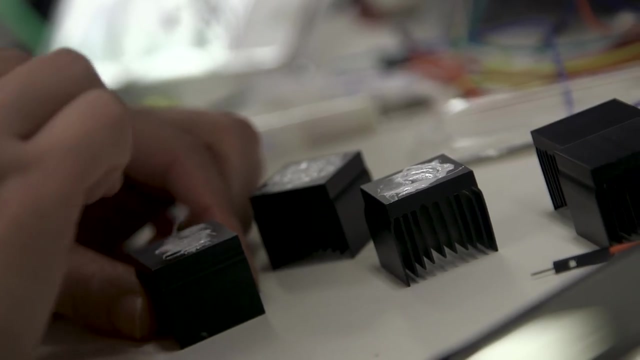 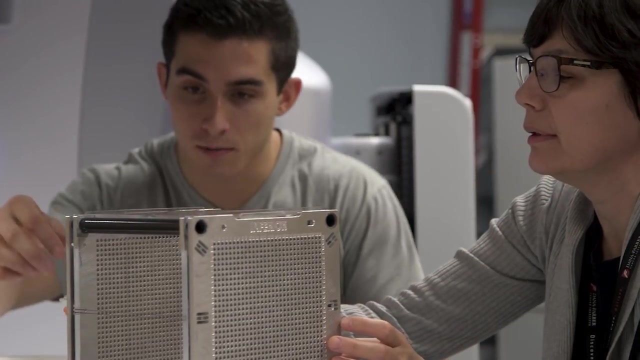 Which is a lot of pressure but an incredibly motivating and enriching experience. Our team worked on building a blue light sterilization device to decrease the risk of surgical site infections. Radio Phantom is a device that's capable of placing radio-opaque markers in 3D space to simulate the topology of a patient's brain lesions. 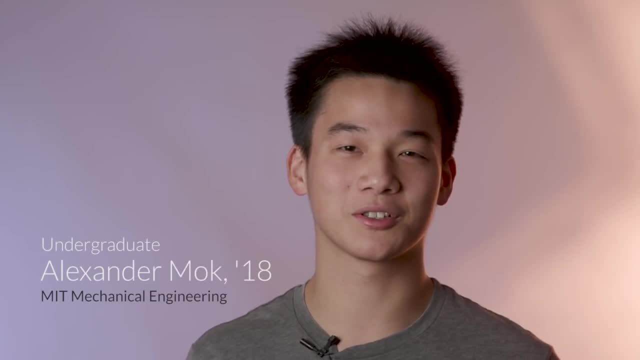 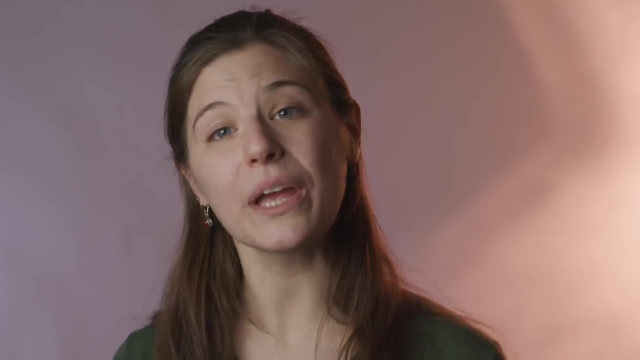 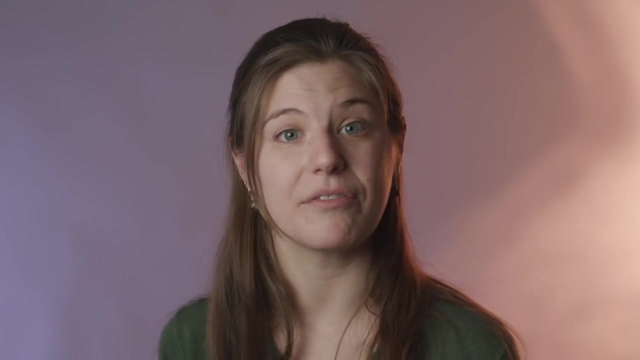 Our wearable device allows elderly patients to more easily and comfortably monitor their cardiorespiratory function. Working with a clinician throughout the project really kept us grounded in the realities of in-home dialysis And how incredibly frightening and painful it can be The ability to actually step foot in the hospital.